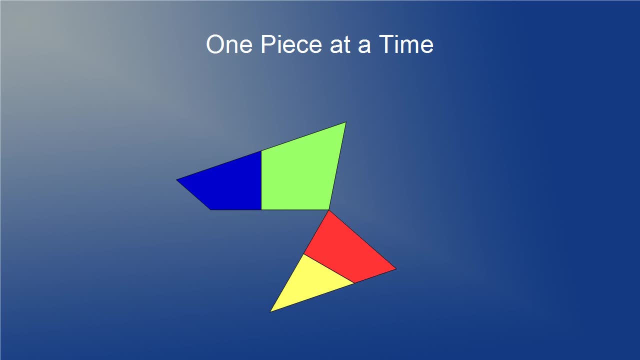 So in this animation you can more clearly see the unfolding of the top pieces down to line up with the bottom pieces and then swing around underneath to complete the triangle. It's easier to trace where the pieces and lines start and finish And it allows us to draw conclusions about where some of the intersections must be and how long certain segments must be in relation to each other. 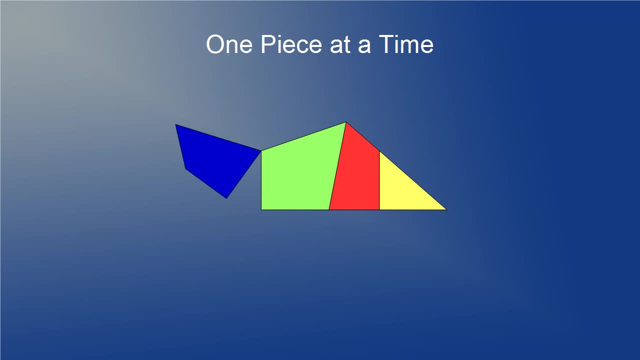 So I'll put up a few problems based on this transition and I think they're a really good exercise for someone studying geometry or trigonometry who wants to use the principles learned in these courses to analyze the structure of this dissection. I'm going to focus on the square for these problems because it's a bit easier to work with. 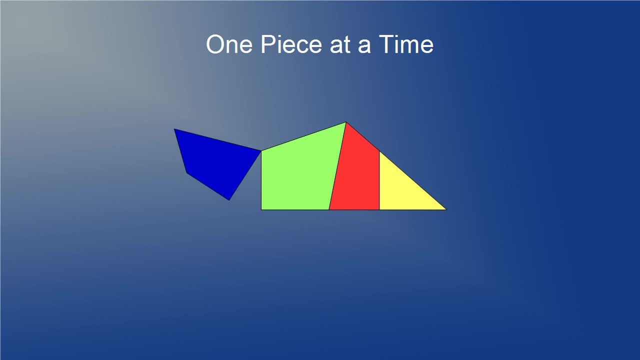 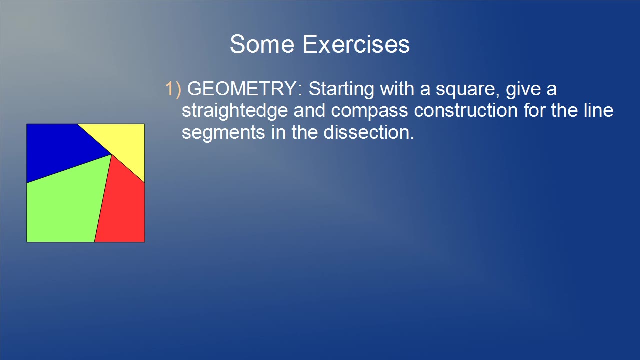 It lines up with the grid on the coordinate plane when you place it at the origin. The first problem is to start with the square and give you Euclidean straight edge and compass construction. for this diagram, The straight edge and compass construction is really the bread and butter of Euclidean geometry. 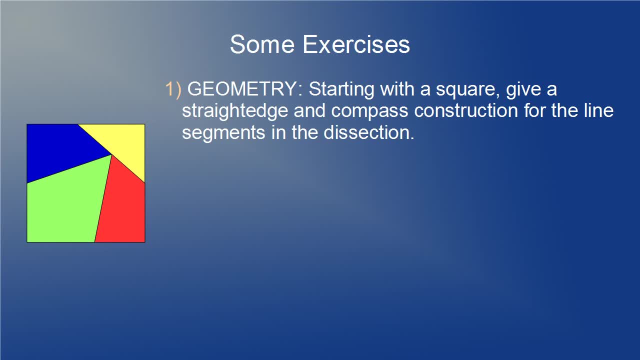 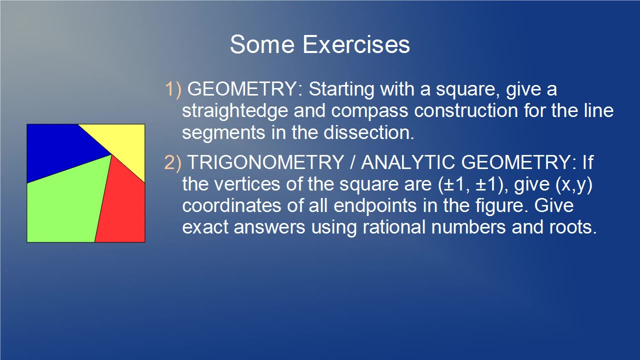 And this dissection is a nice exercise for some basic construction techniques. Secondly, we would like to place the square on the coordinate plane centered at the origin, with the vertices at plus or minus 1,, plus or minus 1, and give x- y coordinates of all the endpoints in the figure. 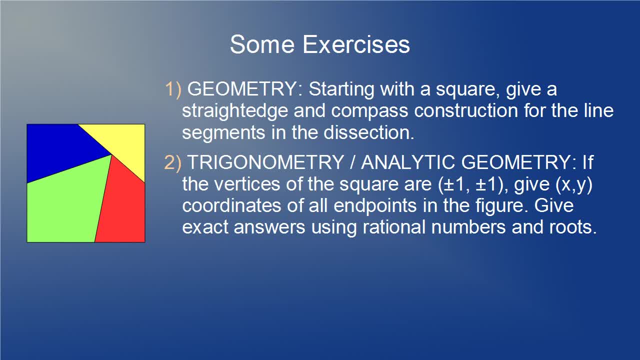 And we'll want exact answers in terms of expressions involving rational numbers and their roots, from which we can compute the decimal approximations. Notice that this is not the unit square. It's a square with side of length 2.. I'm doing it this way because I think it's good to have symmetry about the origin and to have the vertices of the square on the coordinate grid. 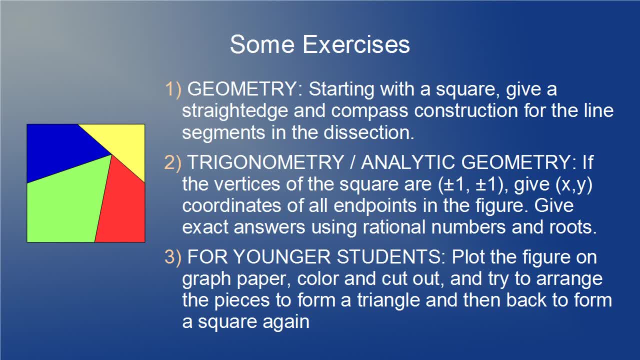 Finally, for younger students or students of all ages, really plot the figure on graph paper, color and cut out and try to arrange the pieces to form a triangle and then back to form a square again. It's a little puzzle that's not that easy. 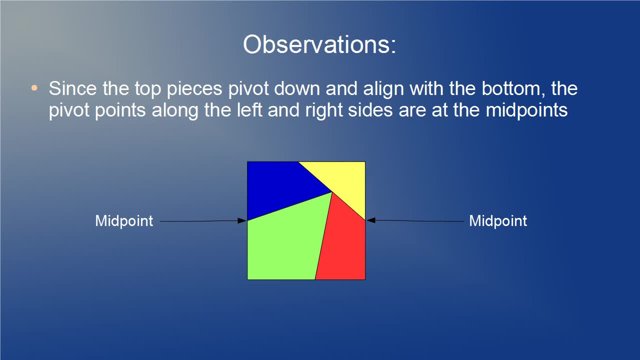 So let's get down to business, And I'm going to start on these problems with some observations, And these observations are from watching the second animation. So observation number one: Since the top pieces pivot down and align with the bottom, the pivot points along the left and the right sides of the square are at the midpoints. 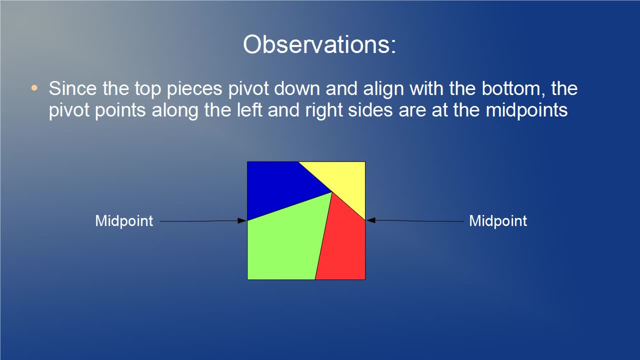 So that's an easy way to start off the answers to any of these questions with two points whose coordinates are easy to determine and describe. Secondly, let's look at that very busy point inside the square- We'll call this point x And notice that the three vertices of the dissected equilateral triangle 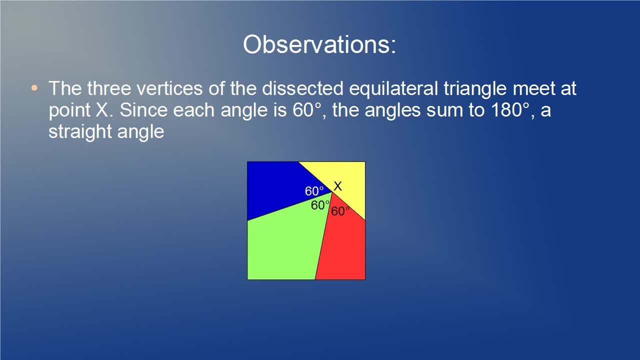 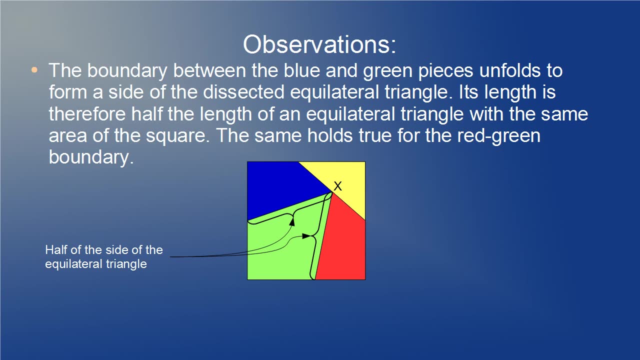 meet at point x. Since each angle is 60 degrees, the angles sum to 180, a straight angle. Another observation is that the boundary between the blue and the green pieces unfolds to form a side of the dissected equilateral triangle. Its length is therefore half the length of an equilateral triangle with the same area of the square. 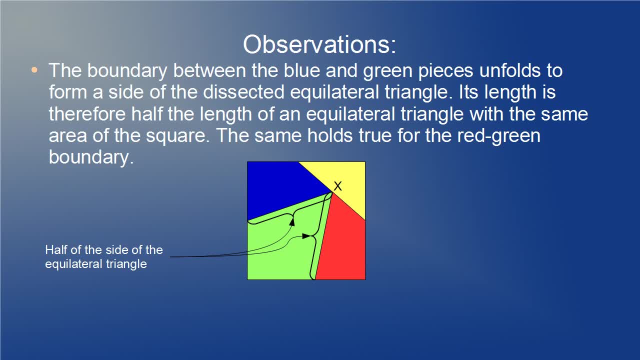 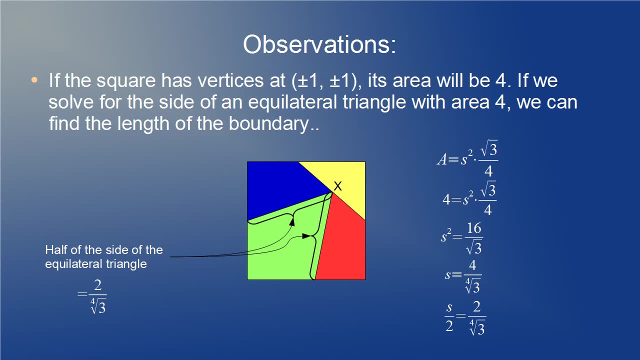 The same holds true for the red-green boundary. The length of those segments are the same. Let's calculate the length of it. If the square has vertices at plus or minus 1,, plus or minus 1,, its area will be 4.. 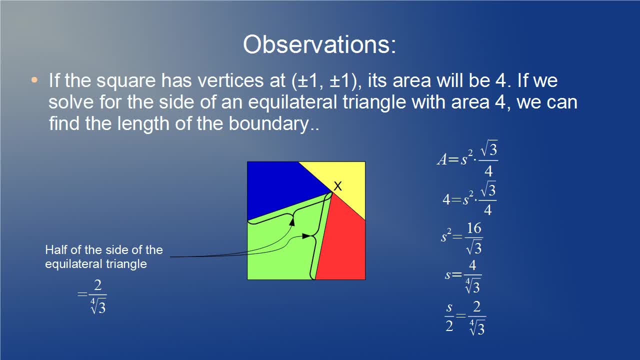 If we solve for the side of an equilateral triangle with area 4,, we can find the length of the boundary between blue and green or green and red. The area of an equilateral triangle, in terms of its side, is s squared times root 3 over 4.. 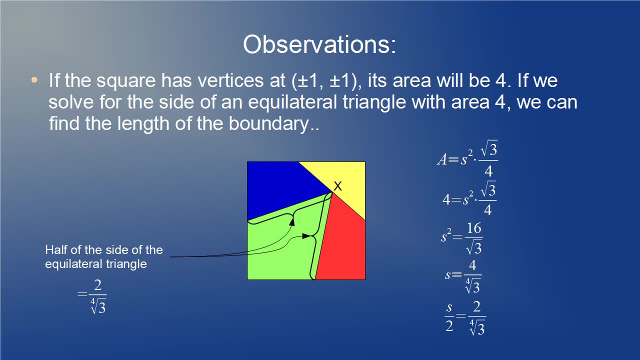 That formula follows directly from using 1 half base times height, where the base is s and the height is s, times root 3 over 2, which you can get in any number of ways, Sine of 60 degrees or better. yet 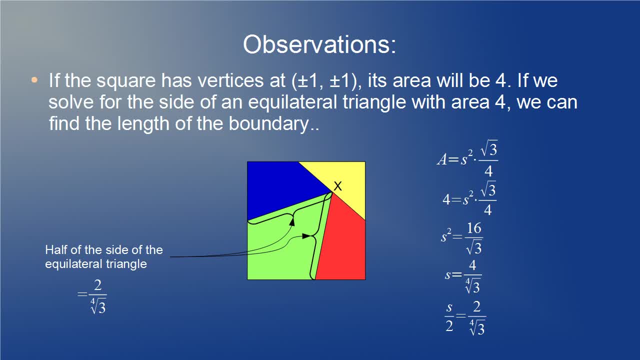 the Pythagorean theorem on a right triangle whose legs are s and s over 2.. Setting s squared root 3 over 4 to the area of our square of side 2, which is 4,, we do some algebra and find that the side s is equal to 4 over the fourth root of 3.. 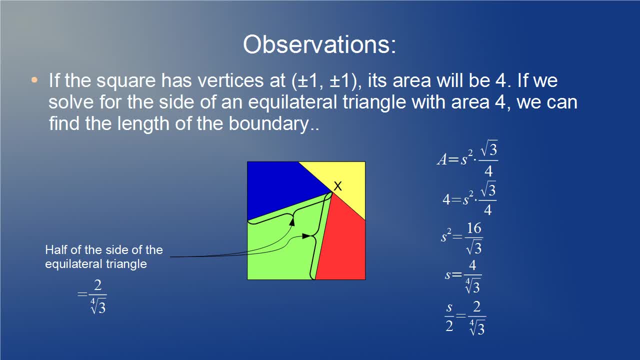 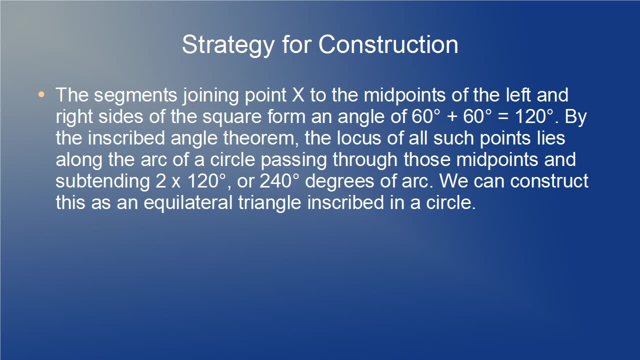 What we really need is half that, since we're looking for the length of a segment that unfolds to that length. So divide by 2 and get 2 over the fourth root of 3.. Now let's form a strategy for the construction based on these observations. 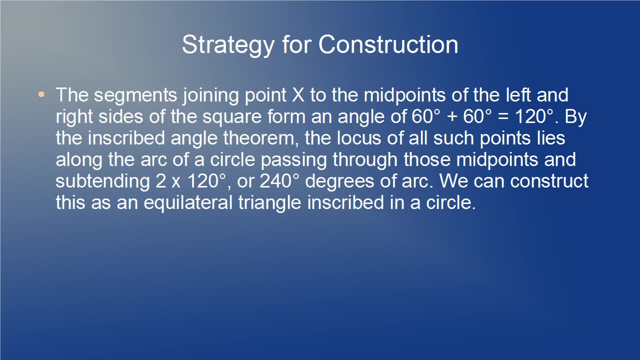 First, the segments joining point x to the midpoints of the left and right sides of the square form an angle of 60 degrees plus 60 degrees, and that's 120 degrees By the inscribed angle theorem. the locus of all such points lies along the arc of a circle passing through those midpoints. 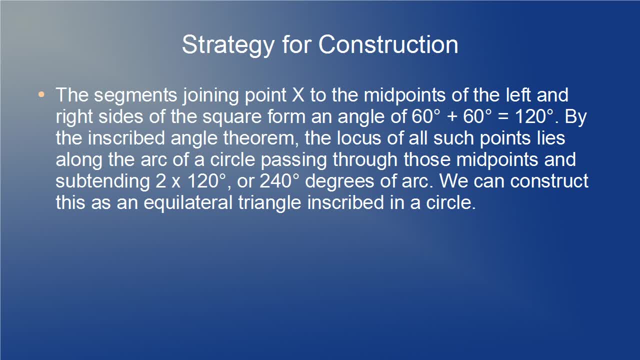 and subtending 2 times 120 degrees or 240 degrees of arc, We can easily construct this as an equilateral triangle inscribed in a circle. Now let's combine this with the fact that the segment dividing the blue and green has length 2 over the fourth root of 3.. 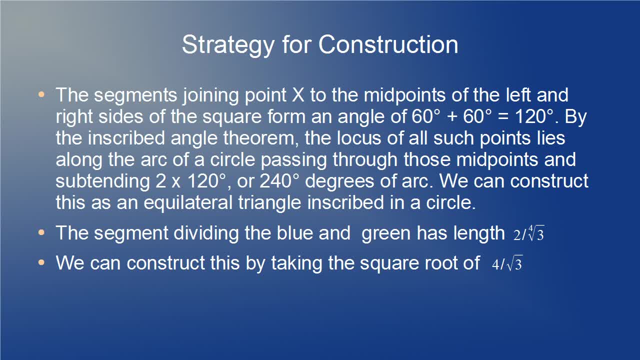 We can construct this by taking the square root of 4 over root 3.. That's an easy length to construct and we get it for free because the diameter of the circle in the previous step has exactly that length. So here we go with the construction. 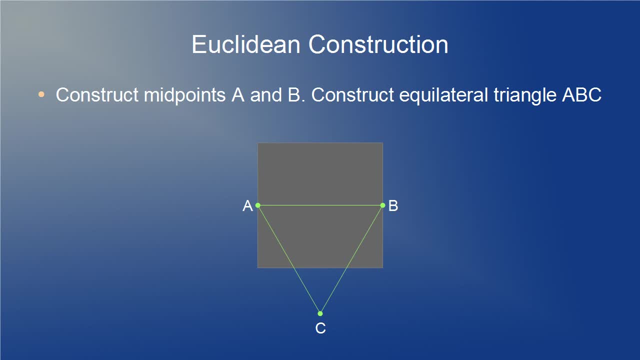 I'll do the current step in green each time to highlight it. Construct the midpoints a and b for the left and right sides respectively. getting the midpoint is an easy basic construction, so I'll omit the details. Next, construct an equilateral triangle with a, b as a base and pointing downwards. 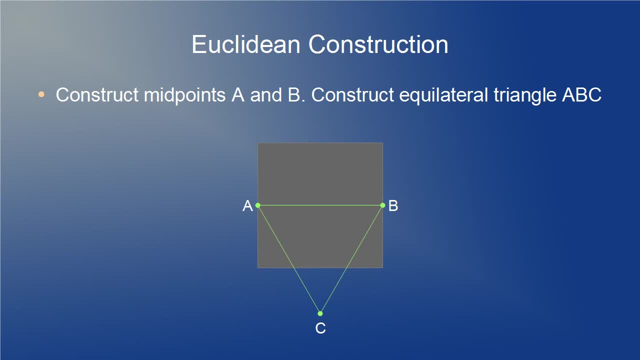 That's an easy construction as well. just set the compass on a, b and make little arcs with centers a and then b that intersect at the vertex c. Next, circumscribe a circle around this equilateral triangle. You can find the center by intersecting angle bisectors. 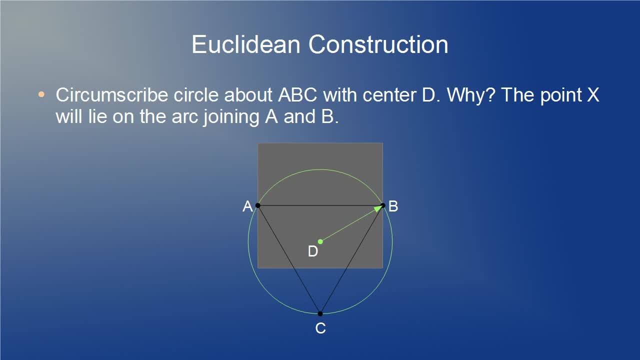 It's elementary so I won't show you those details. We've done this because the point x will lie on the arc a- b in the upper rectangle. You can take any point on that arc as long as it's strictly between a and b. 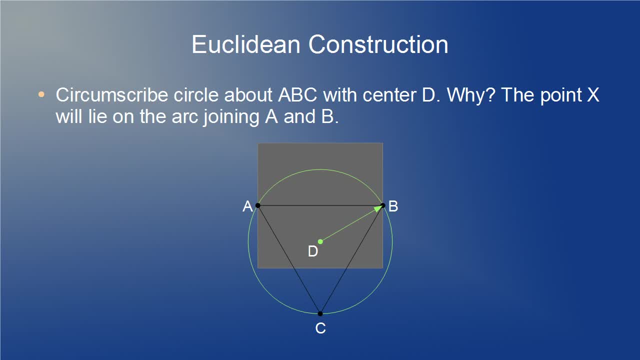 Draw segments directly to a and b and the angle will be 120 degrees, no matter where on that arc you choose. Moreover, if you draw the line to c, you'll bisect this angle and get two 60 degree angles, and we'll do exactly that later on in the last step, since we need that segment. 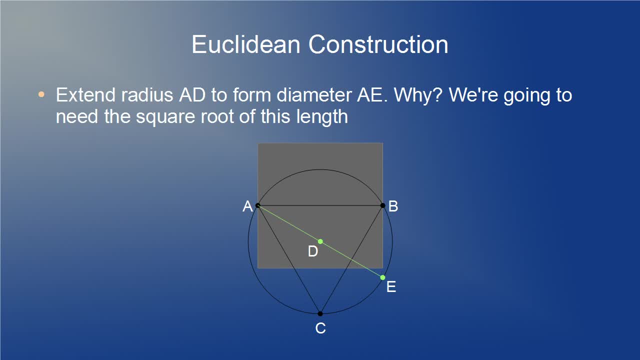 Next, let's extend the diameter a e. As mentioned, a e will have length 4 over root 3, and if we can take the square root of this, we'll have the length between a and x, which is the final piece of information we need to construct x. 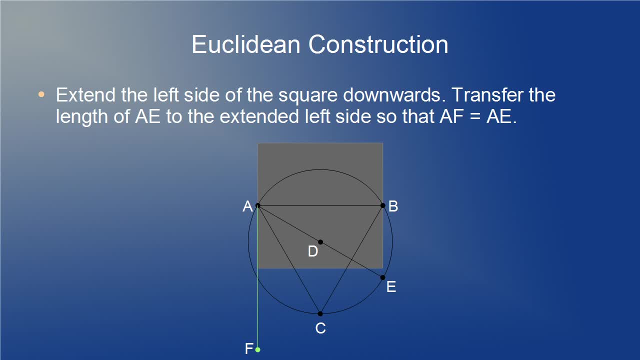 For the square root construction we need to add a segment of length 1 to the segment a e, and that will be done by transferring its length to an extension of the left side, as shown at a f. Then the next step in the square root construction will involve bisecting the segment g f at h. 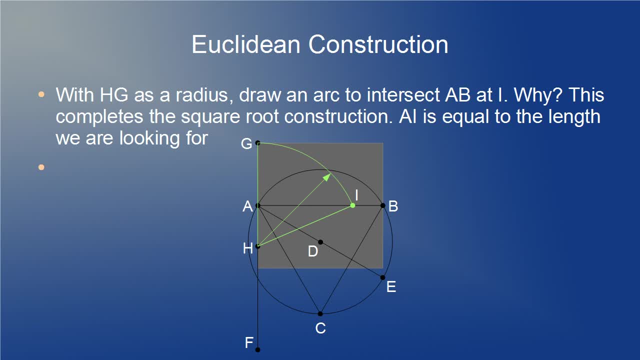 Then with h, g, f, draw an arc to intersect a- b at i. This completes the square root construction and a- i is equal to the length between a and x, which is 2 over the fourth root of 3.. To find x, then, we just need to take a- i as a radius. 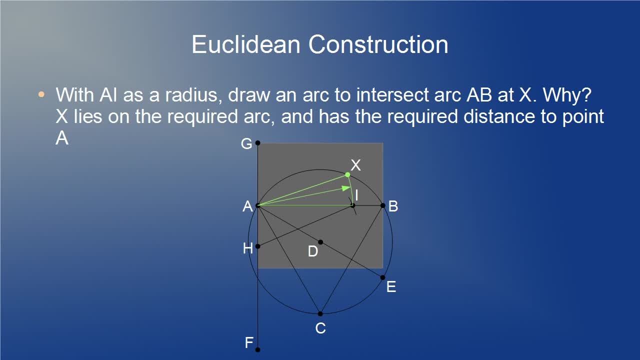 and draw an arc to intersect the arc a b at x. This has to be our point, since it's the only point with the required distance to point a and it lies on the arc which will guarantee that angle a x b is 120 degrees. 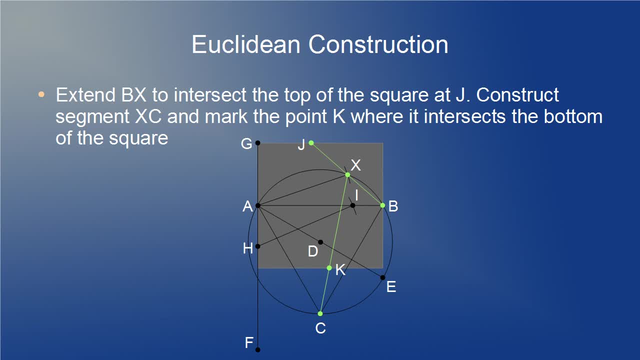 To complete the construction with all required segments, simply extend b- x to the top of the square at j and for the bottom segment, construct segment x c which by the inscribed angle theorem will bisect the 120 degree angle a x b. 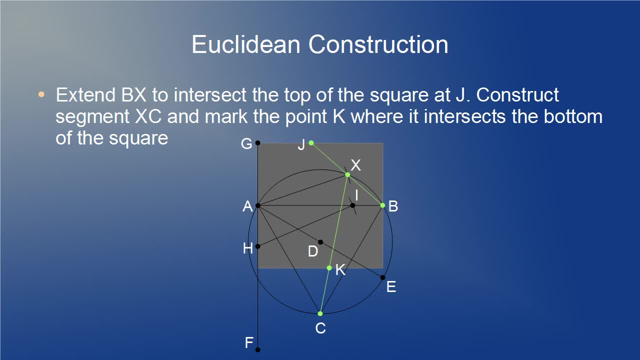 into a pair of 60 degree angles, as required. I'll just remark at this point that this is not the only possible construction, of course, and it may not even be the best construction, depending on your criteria. This construction was actually my second attempt. 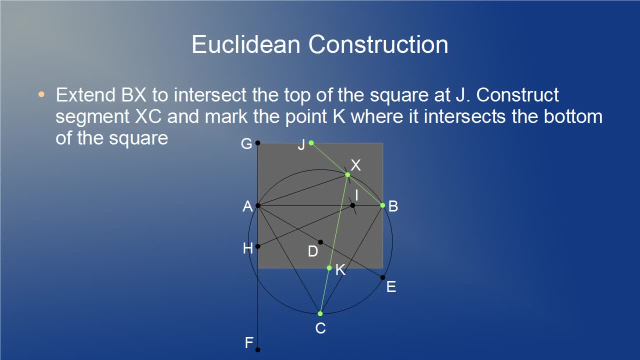 my first attempt was to construct the segment c, k, x. by constructing the small angle x, c, d that it makes with the vertical, You can actually find a quadratic expression for the tangent of that angle. solve the quadratic and construct the angle. This took quite a few more steps, so I found a cleaner construction in the one presented. 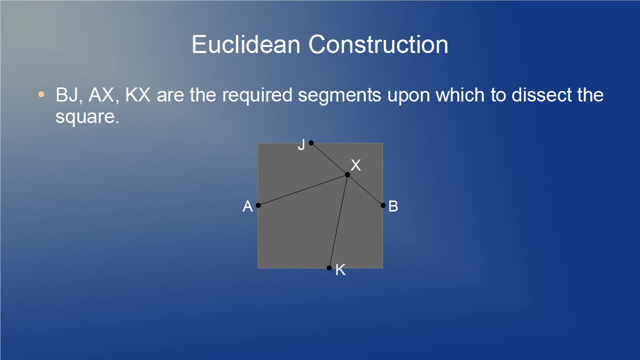 Now in the final slide, we'll get rid of the unused construction lines and show the required segments upon which to bisect the square. and those are the required endpoints. The next problem involves finding the Cartesian coordinates of the points a, b, j, k and x. 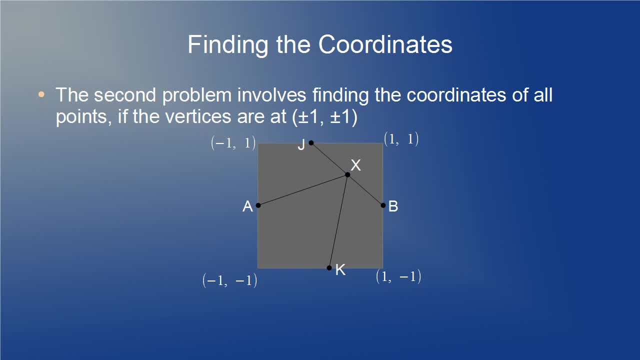 if we place the vertices of the square at plus or minus 1,. plus or minus 1, as shown. As we remarked earlier, a and b are easy. They are the midpoints of the respective sides and lie along the x-axis at and. 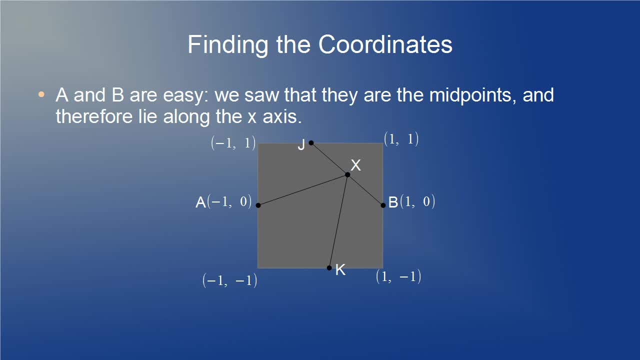 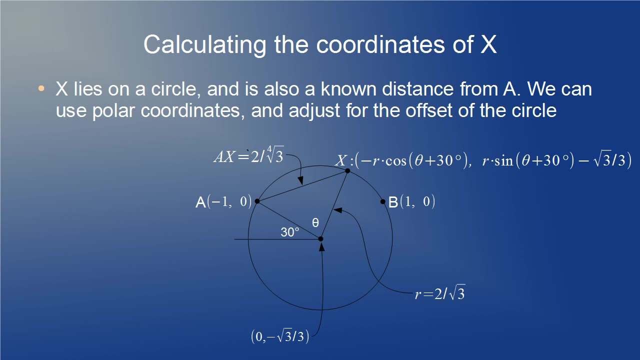 x is going to be a little harder. So the approach I would like to use to find x is to bring back the circle from the Euclidean construction, because the center of that circle makes a nice isosceles triangle with a and x along the circumference. 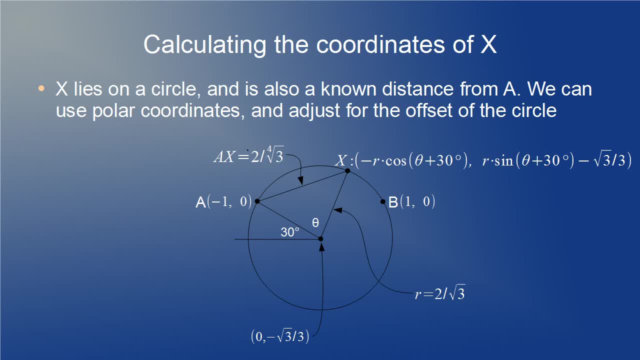 It's also tilted 30 degrees from the horizontal because of the equilateral triangle that was constructed first. So by polar coordinates and adjusting for the offset of the center of the circle from the origin, we get a formula for the coordinates of point x. 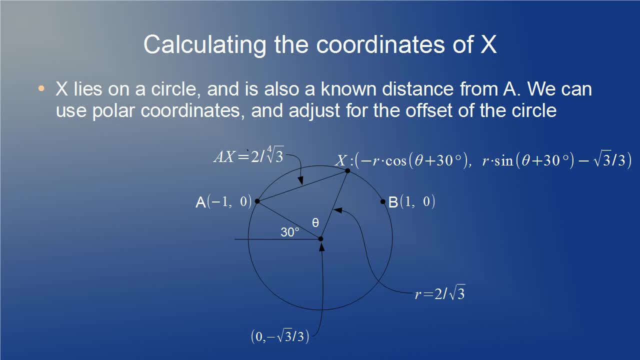 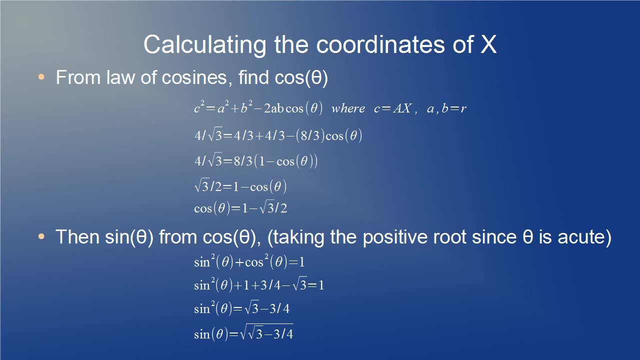 Now we can use some trigonometry to simplify the sine and cosine of those angles. We can find theta, because we have all three sides of the triangle. Two of those sides are radii of the circle and the other is a segment ax. The law of cosines is basically an extension of the Pythagorean theorem. 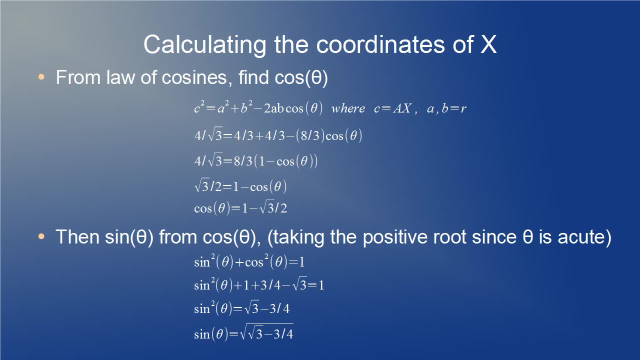 We have a squared plus b squared equals c squared, and then a correction of minus 2ab cosine theta, when the angle is not a right angle. So after a little algebra we find cosine theta is 1 minus the square root of 3 over 2.. 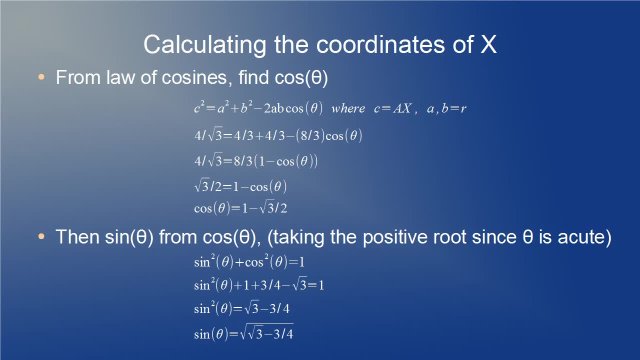 Then sine theta follows from cosine theta. by using sine squared plus cosine squared equals 1. The Pythagorean theorem is at the heart of that equality as well, And we take the positive square root for sine theta, since the angle is acute, And now we have a more complex expression involving two square roots. 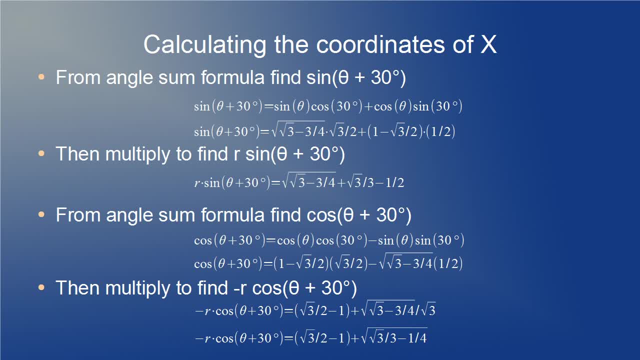 Since these angles are offset by 30 degrees, we can use the sum of angles formula to find sine and cosine of theta plus 30. Sine first Sine of a plus b is sine a, cosine b plus cosine a sine b. So substituting what we just found along with sine 30 equals a half. 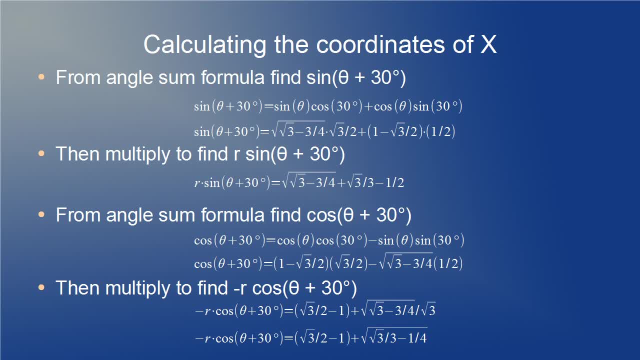 and cosine 30 equals root 3 over 2, we get an equation that resists further simplification. So let's move to the next step and multiply by r, which is 2 over root 3. And that's fortunately going to cancel out some of the root 3 over 2 factors. 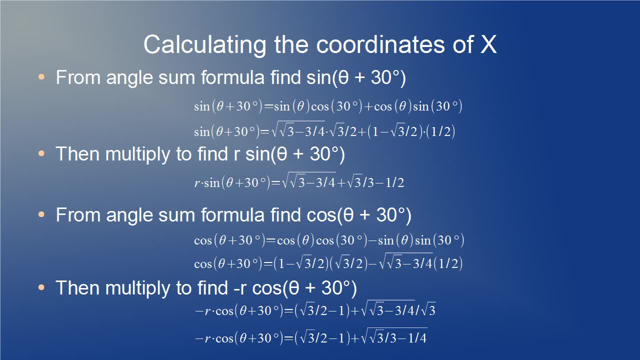 Now to do the same with cosine a plus b. it's cosine a, cosine b minus, sine a, sine b. So again we get an equation that resists further simplification. Again we can multiply by r, which is 2 over root 3,. 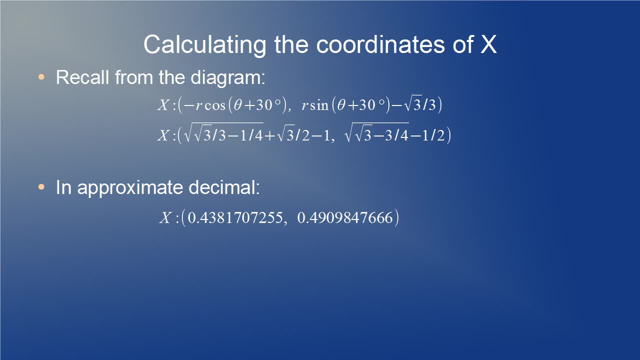 and get some cancellations. So let's collect these results and express as coordinates. for x, We need to subtract root 3 over 3 to account for the offset of the circle from the origin, and this fortunately cancels an equivalent term. So we have the expression as shown. 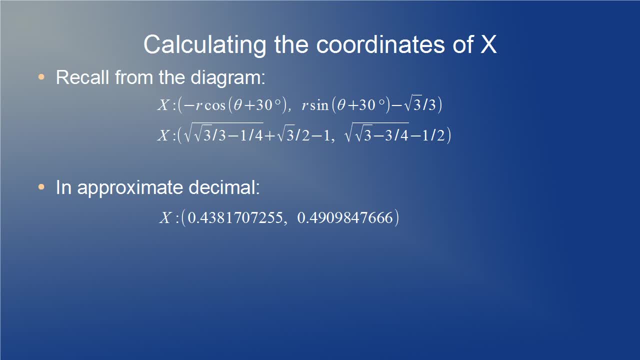 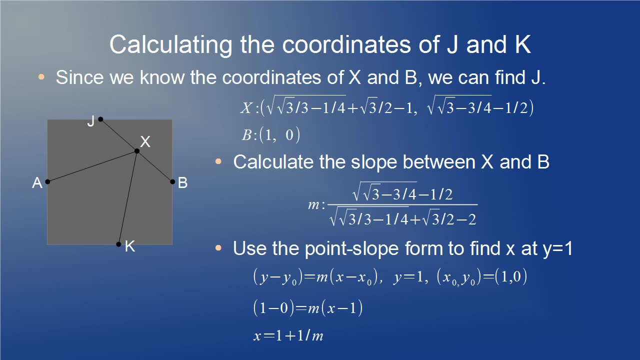 and by converting to an approximate decimal, we see that this is about where we would expect it, near the center of the first quadrant. So the sanity check passes. Now we're left with j and k, Since b, x and j lie on a line. 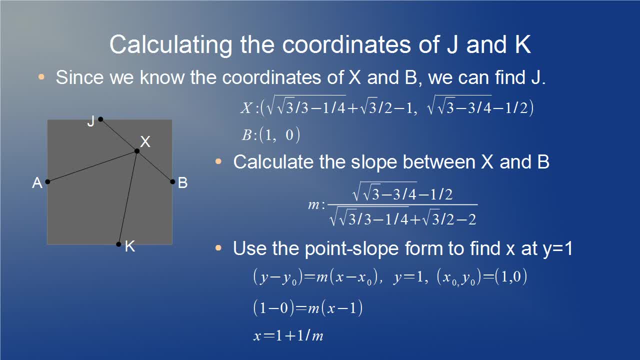 we can use the point-slope formula to find j. Let's first calculate the slope between b and x, That's just delta y over delta x, and we get a monster fraction as shown. Let's just use m to represent that for now. 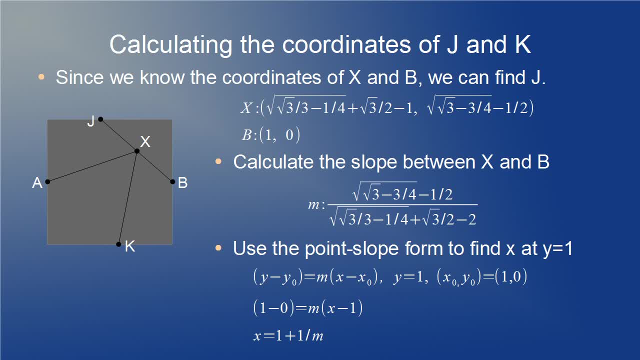 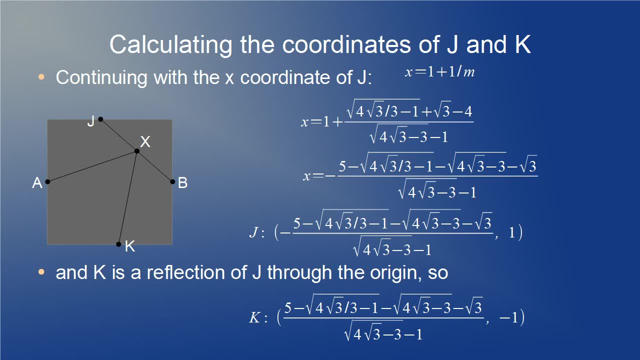 and substitute y equals 1 because j lies along the top of the square, We'll find x equals 1 plus 1 over m. and let's bring m over and simplify. We've gotten rid of the fraction and we've taken the fractions in the numerator and denominator. 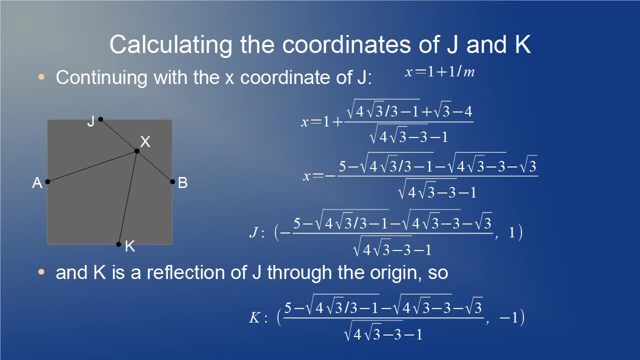 by multiplying each by 2, and then we've taken the reciprocal. In the next step, I've put a negative sign in front and negated the numerator to make it more obvious that the slope is negative. Now we have an expression for the point at j. 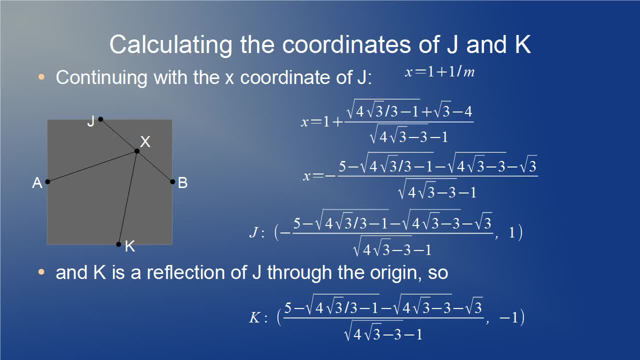 Now we can take a shortcut for k. It's actually a reflection of j through the origin. When the pieces are rearranged, the segments extending left from j and k are joined end-to-end, and the pieces extending right from j and k are also joined end-to-end. 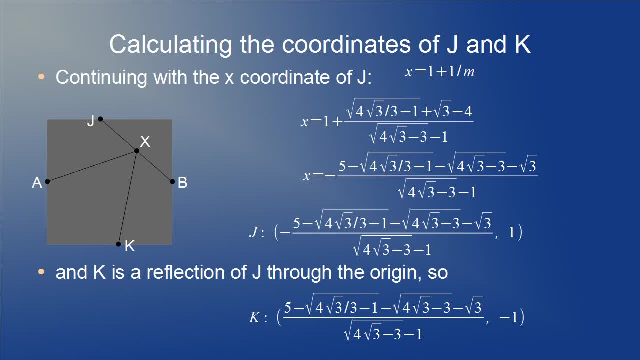 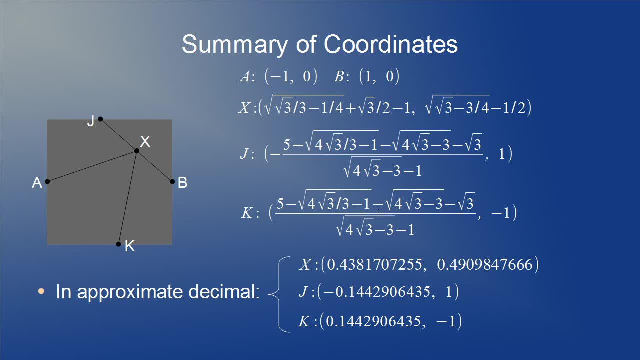 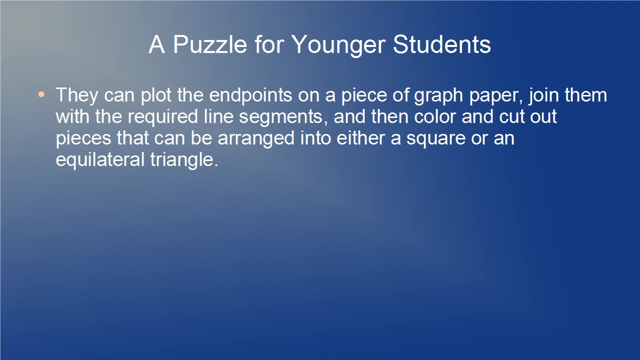 and these resulting segments are superimposed, so they must have the same length. This requires that j be a reflection of k through the origin, so k follows from j simply by negating both coordinates. Now let's go to that final puzzle for elementary school students. 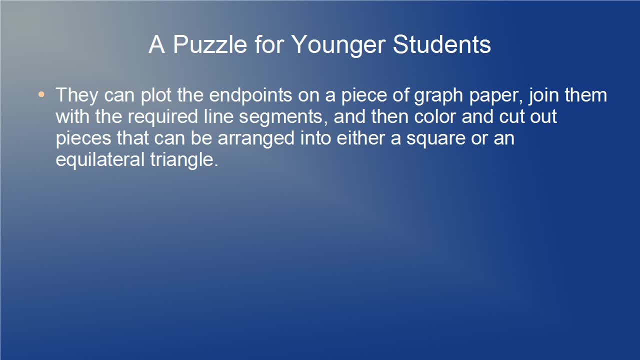 We would like them to plot the points on a piece of graph paper, join them with the required line segments, then color and cut out pieces that can be arranged into either a square or an equilateral triangle. Now that we know the coordinates of the points. 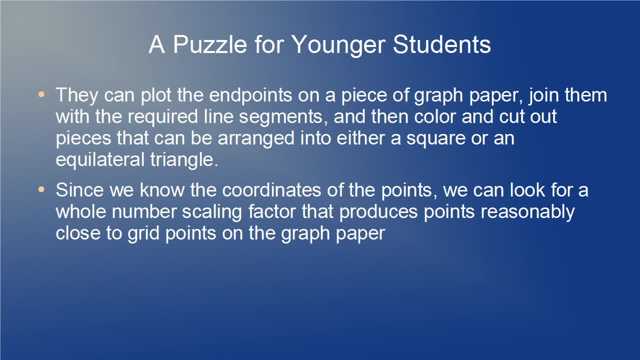 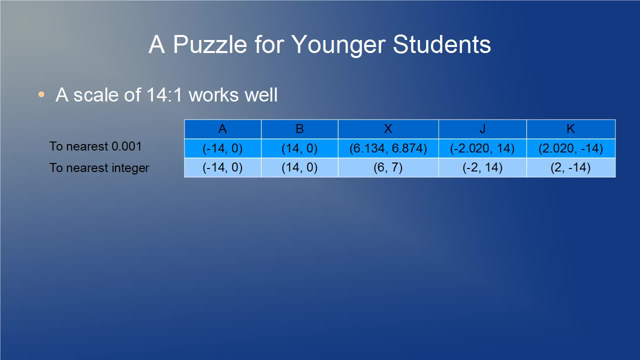 we can look for a whole number scaling factor that produces points reasonably close to grid points. on the graph paper, A scale of 14 works well, as you can see in the chart. here, j and k are quite close. x needs just a bit more rounding, but nothing too extreme. 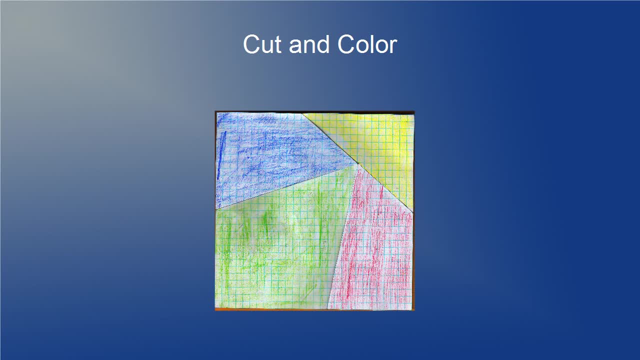 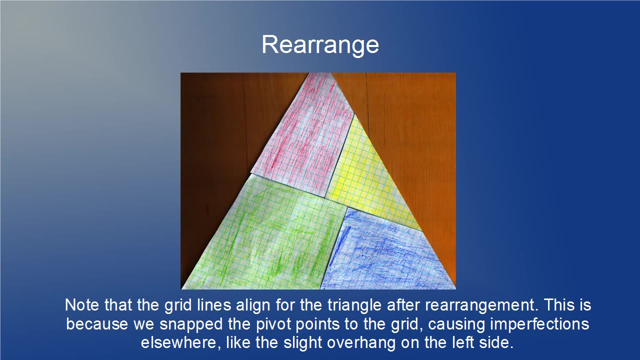 Now here's what it looked like when I cut it out and colored it and, upon rearrangement, I was surprised to see that the grid lines align for each piece. This is because we snapped the points together and the pivot points to the grid. 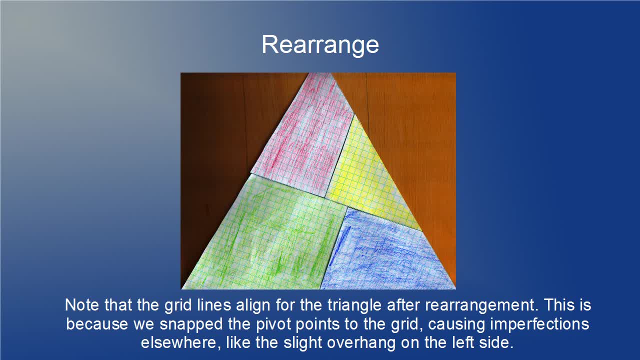 And the pivot point at k is not actually on the grid, so the lines should be offset a bit. We've got a little bit of imperfection with the overhang on the left, as you can see, but nothing too extreme. We should ask some questions to help the students learn. 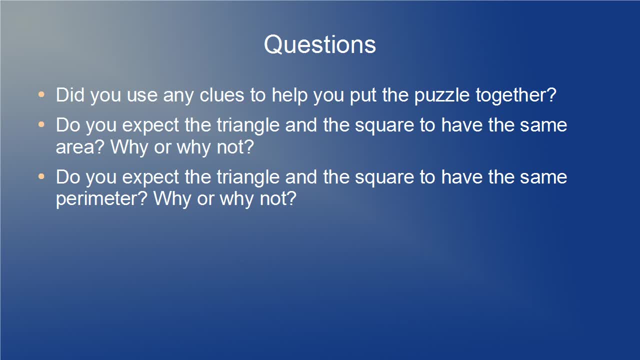 For instance, did you use any clues to help you put the puzzle together? Do you expect the triangle and the square to have the same area- Why or why not? And do you expect the triangle and the square to have the same perimeter- Why or why not? 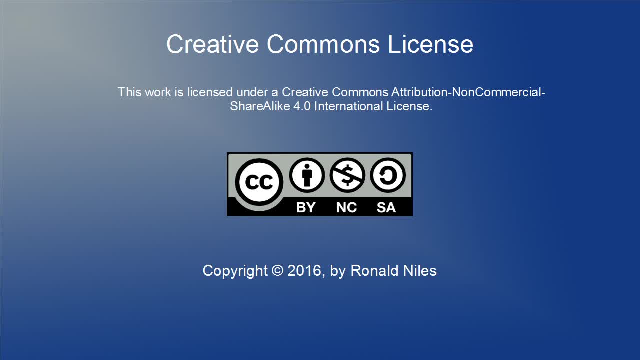 So, once again, thanks for watching. I hope you learned something from analyzing this interesting transformation. I know I did. 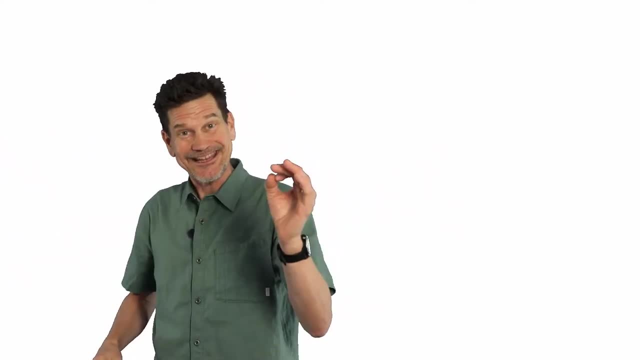 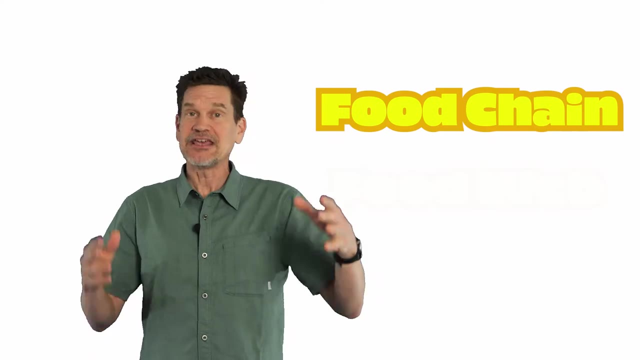 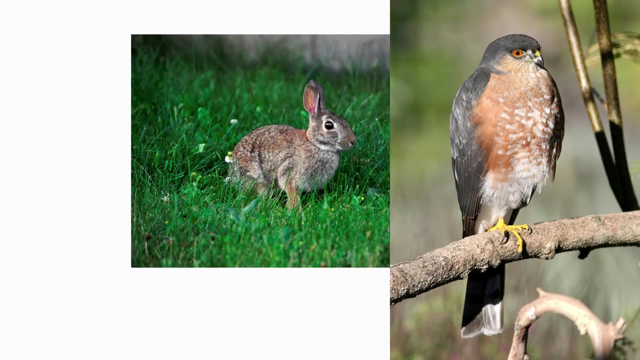 Hello and welcome to Speaking Scientifically. Today we're going to look at the difference between a food chain and a food web. A food chain is a map of who eats who. For example, a hawk might eat a rabbit, the rabbit might eat some grass and the grass makes its own food using. 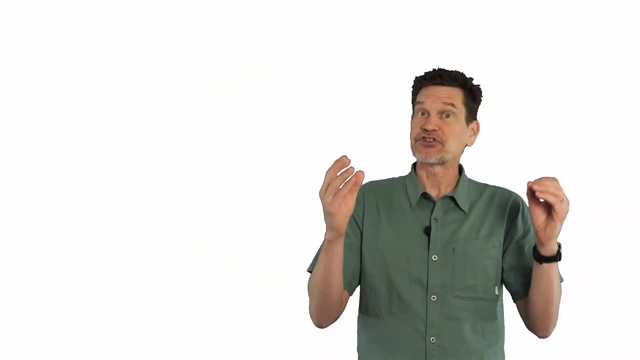 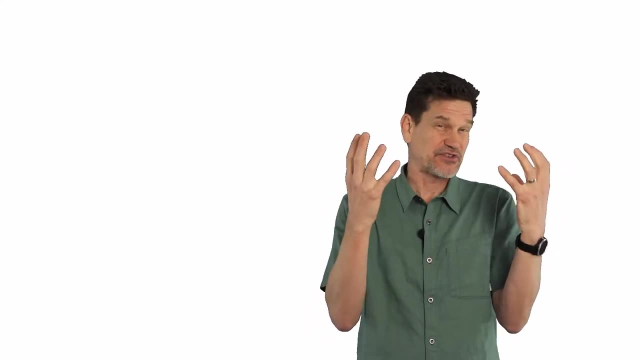 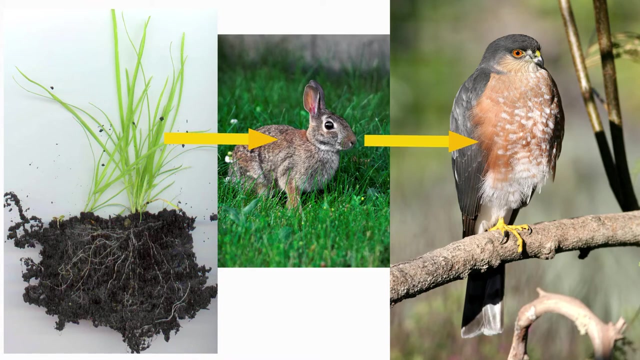 energy from the sun. Now, the real lesson you're supposed to learn from a food chain is that plants are the producers, and the energy from the sun that they capture gets passed on to the herbivores and then passed on to the carnivores and omnivores, so that almost all life on earth is ultimately 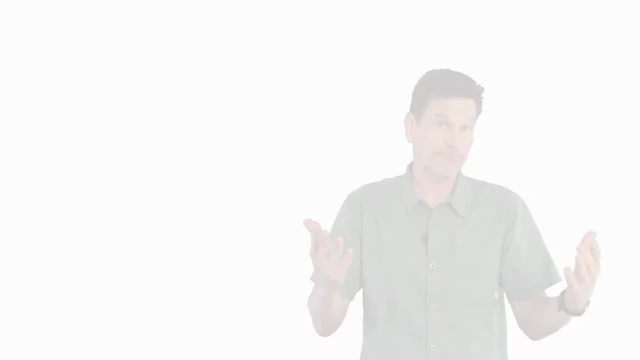 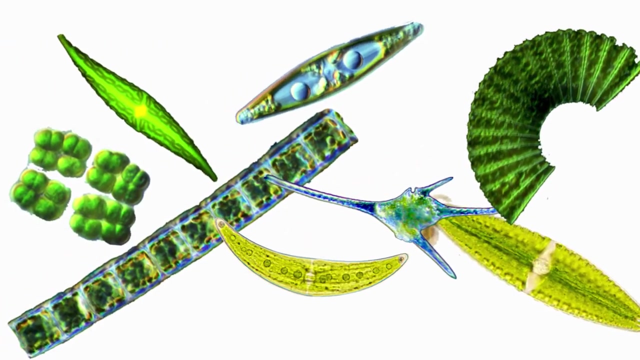 powered by the solar energy that plants capture In the ocean. the producers are mostly these single-celled animals that produce energy from the sun. The plants are the producers, and that's algae dudes called phytoplankton. Like plants, they produce food using solar energy. 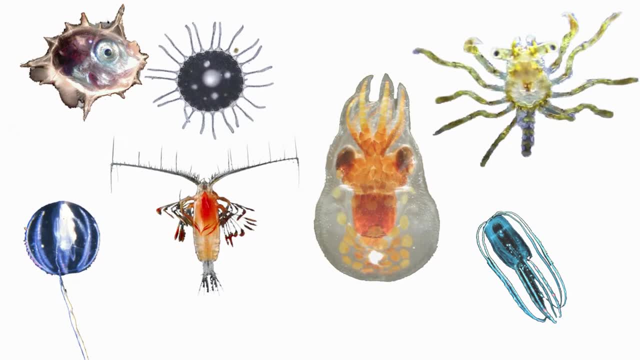 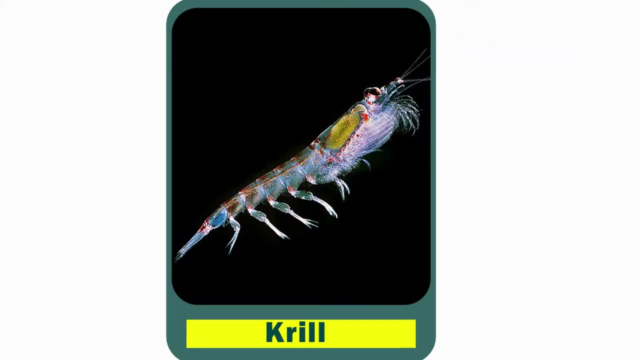 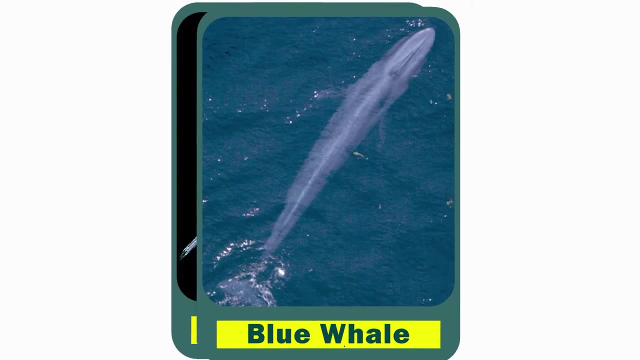 The phytoplankton are often eaten by the animal kind of plankton called zooplankton. A krill is a very famous kind of zooplankton because they get eaten by Earth's largest animals, the blue whale. So there's an ocean food chain. A blue whale eats krill and krill get their energy. 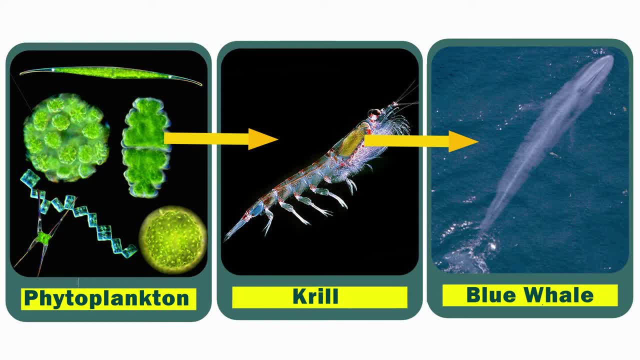 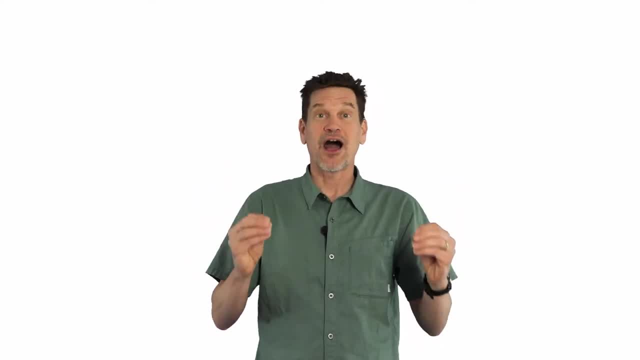 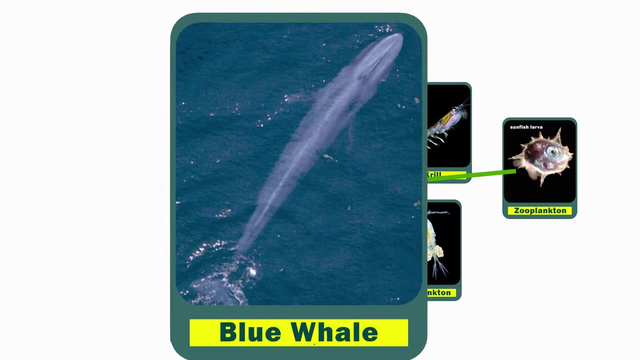 from the phytoplankton, and the phytoplankton get their energy from the sun. Now a food web shows that it's a lot more complex than this. Zooplankton don't just get eaten by whales- right Clams eat zooplankton.